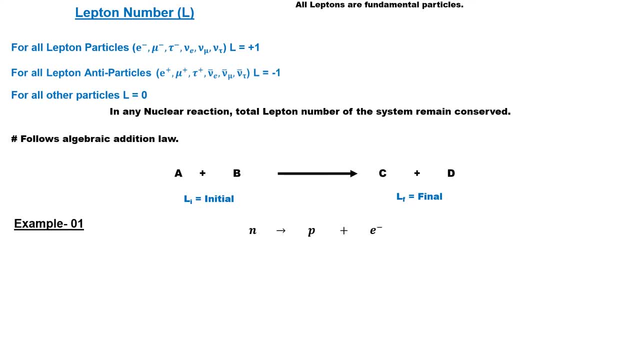 into proton and electron In this decay. proton and neutron are non-leptonic particles, So their lepton number will be zero, while electron is a lepton particle, so its lepton number will be plus one. Since lepton number is not conserved in this reaction, therefore, this reaction is forbidden. 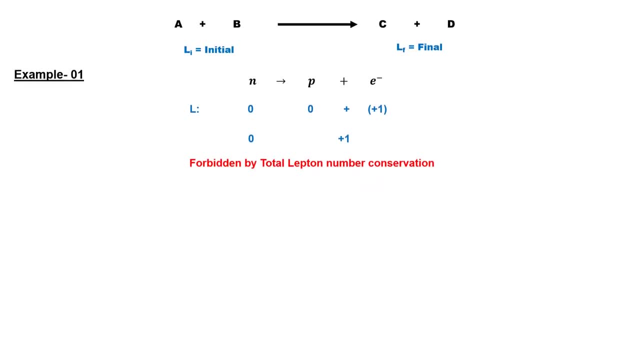 according to lepton number conservation, The neutrino is decaying into proton, electron and antineutrino. Since antineutrino is an anti-lepton particle, so its lepton number will be minus 1.. In this BK reaction the lepton number is conserved, so this reaction is allowed according. to lepton number conservation. After the discovery of lepton number, some reactions were conserving lepton number, but still that reaction was not allowed. Like muon, neutrino and neutron being decay into electron and proton, This reaction has neutrino and electron lepton particles, hence their lepton number will. 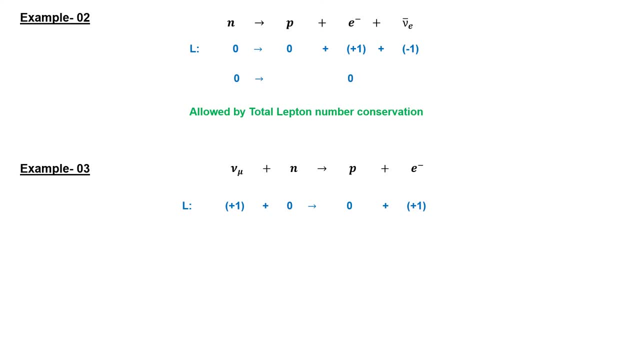 be plus 1, while neutron and proton are non-leptonic particles, so their lepton number will be 0. So, even though the lepton number is conserved in this reaction, but still the reaction is not allowed To resolve this problem, all lepton particles were divided into lepton flavor or lepton family. 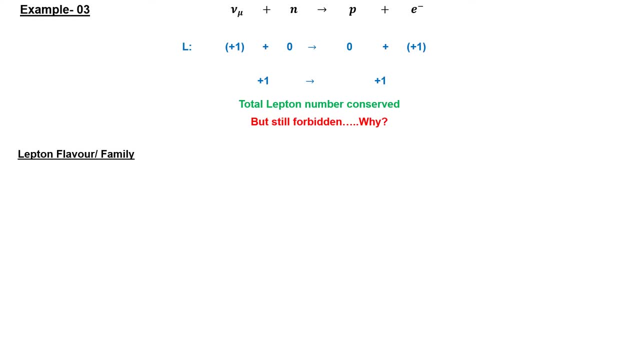 All six leptons are divided into three families. The electron family has members electron and electron neutrino. muon family has members muon and muon neutrino. and tau family has members tau and tau neutrino. For all these families a new quantum number were defined. 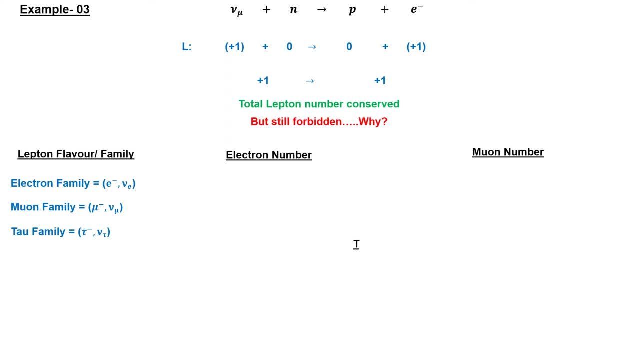 Like electron number for electron family, muon number for muon family and tau number for tau family. This is defined as plus 1 for particles, while minus 1 for antiparticles in each family. If a lepton particle belongs to another family, that lepton number of this family will be. 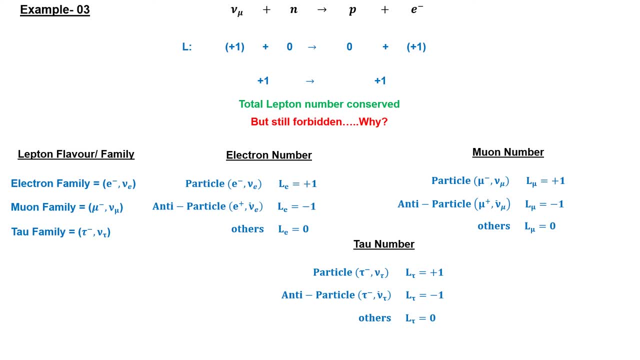 0 for that. Now, according to lepton number conservation, any nuclear reaction can be allowed only when total lepton number as well as lepton number in each family are conserved. So this reaction can be allowed only when total lepton number as well as lepton number. 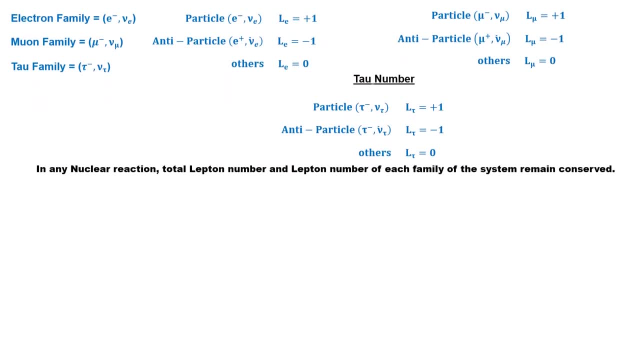 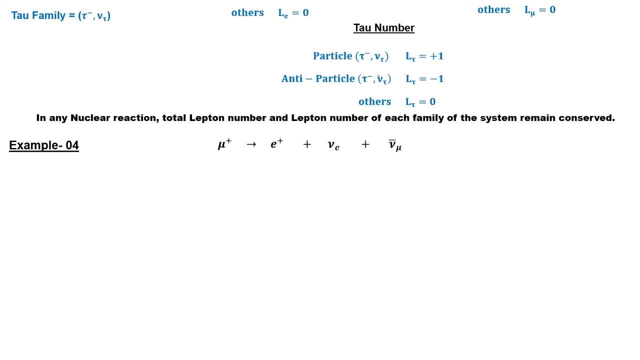 in each family are conserved. Let us understand this with an example Such as muon decays to positron, electron neutrino and antimuon neutrino. In this reaction, neutrino is a lepton particle, so its lepton number will be plus 1, while 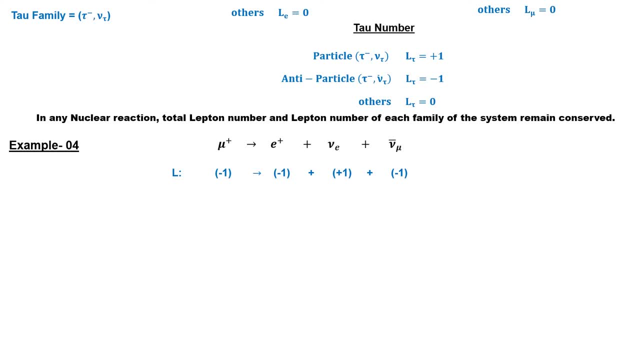 muon, positron and antineutrino are antilepton particles, so their lepton number will be minus 1.. In this way, the total lepton number is conserved in this reaction. Talking about lepton number to be conserved in each family, let's first verify electron. 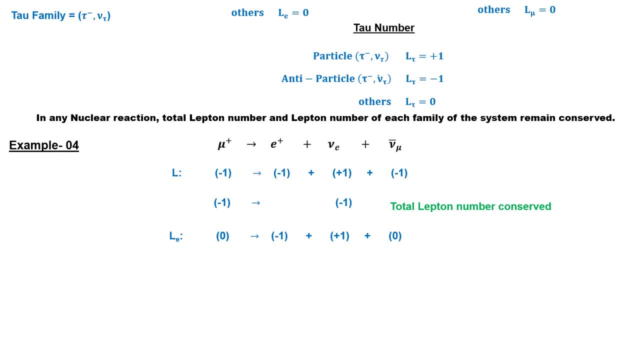 number, Then positron and electron neutrino are the members of electron family, while the muon and antimuon are not the members of electron family. In this way, electron number is also conserved in this reaction. Talking of muon number, muon and antimuon neutrino are members of muon family, while positron, 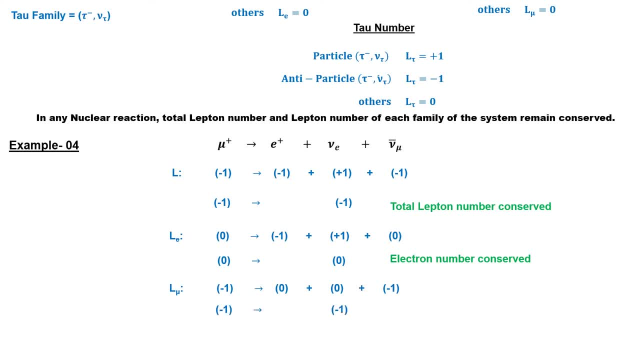 and electron neutrino are not. They are not conserved. Therefore muon number is also conserved, Since in this reaction the total lepton number as well as the lepton number in each family is conserved. therefore this reaction is allowed. 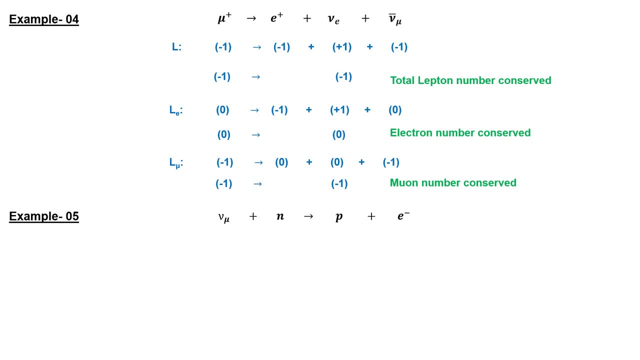 If muon, neutrino and neutron are decay into electron and proton, then total lepton number is conserved in this reaction. But if we talk of electron number, then in this reaction electron is the only member of this family. Because of this, 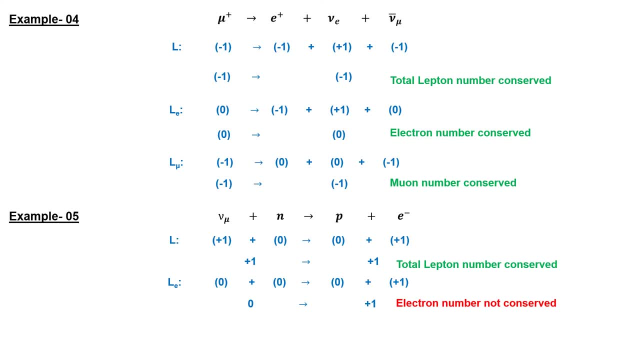 In this case, the electron number is not conserved. Similarly, muon is the only member of muon family in this reaction. Therefore, the muon number is also not conserved. Kion is decaying into pion and electron. 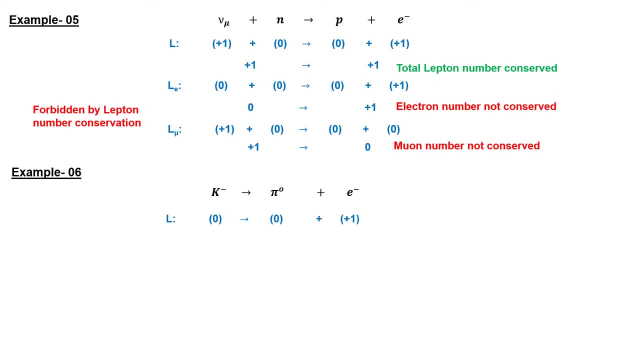 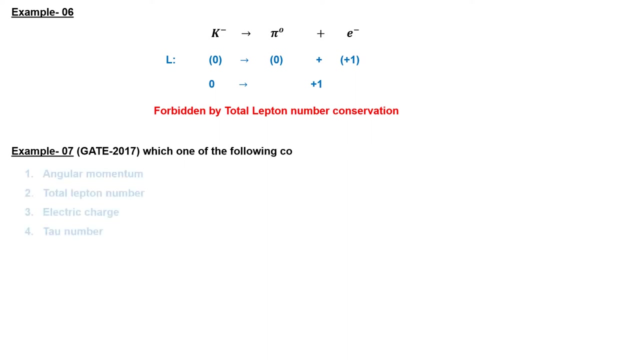 In this reaction, electron is a lepton particle, while kion and pion are non-leptonic particles. Since total lepton number is not conserved, therefore, this reaction is a violation of total lepton number conservation. In GATE 2017,, it was asked which one of the following conservation law is violated in: 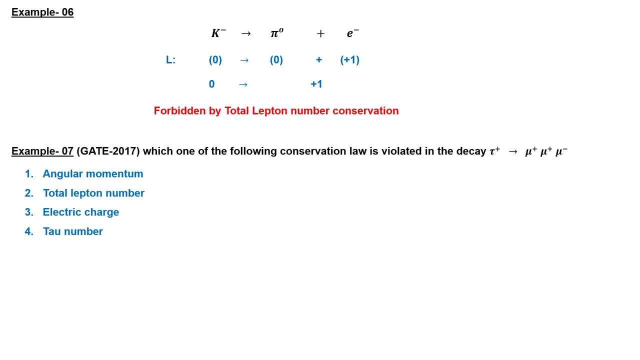 this decay. In this decay reaction, total lepton number is conserved, but tau number is being violated. Let us first verify the total lepton number conservation In this reaction. muon- is a lepton particle having lepton number plus 1, while tau plus 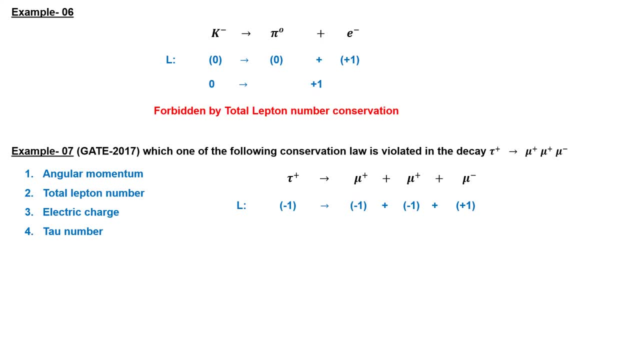 and muon plus are anti-lepton particles having lepton number minus 1. So since total lepton number is conserved, this reaction is allowed according to lepton number conservation. Talk about tau number. In this reaction, tau plus is the only member of tau family. 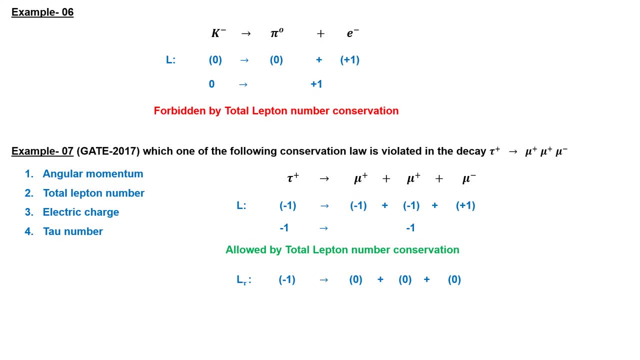 Since muon is not a member of tau family, therefore its tau number will be 0.. As we can see, tau number is not conserved in this decay reaction. Next universal conservation law is baryon number conservation. Lets see how to use this conservation law and how to use this baryon number conservation. 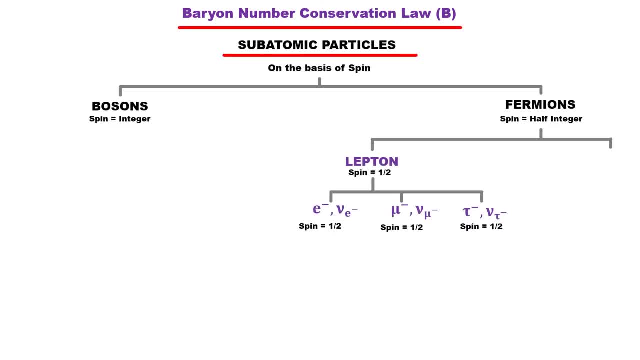 The solution for this is given in the above video of subatomic particles. we know that fermions that interact with strong nuclear force are called baryons. Due to the considerable variation in the mass of baryons, they have been divided into two parts: Light mass baryons are called nucleons and heavy mass baryons are called 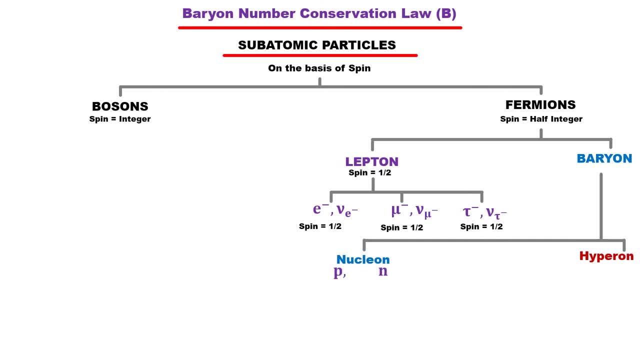 hyperons, So far two nucleons, proton and neutron, while lambda sigma cascade, omega and delta baryons have been discovered. Only omega- and delta baryon have spin 3x2, while rest of the other baryons are fermions of spin 1x2.. Here, one thing to be note is that 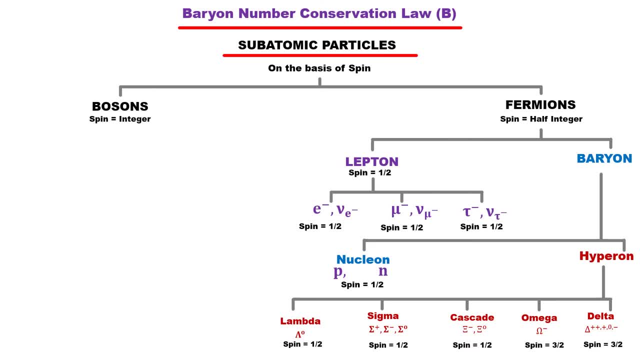 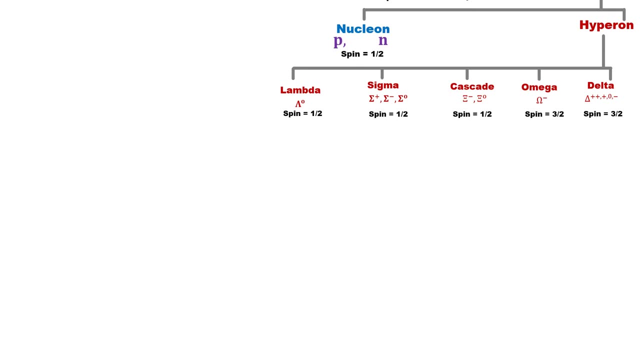 these all are baryon particles. Unlike the meson, sigma- is not the antiparticle of sigma+. rather, these all are particles and their antiparticles are represented by placing a bar over them, Like lepton particles. a special quantum number has been defined for baryon particles. 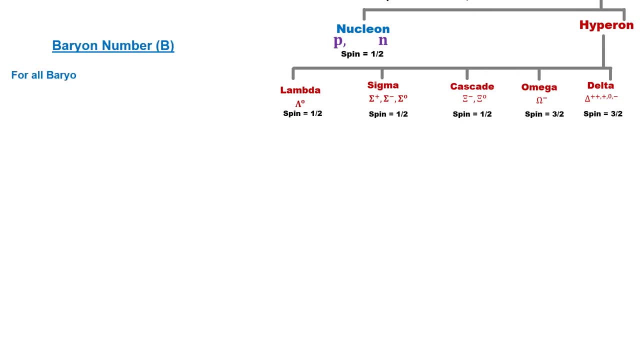 which is called baryon number. For all baryon particles, baryon number is plus 1, while for all antibaryon particles baryon number is minus 1.. Particles which are not baryon have their baryon number 0.. Like lepton number, baryon number also follows algebraic addition. law. According to baryon number conservation, baryon number should be remained constant. baryon number should be remained conserved in any nuclear reaction. If parent particles decay into daughter particles, then the total baryon number of the parent particle should. 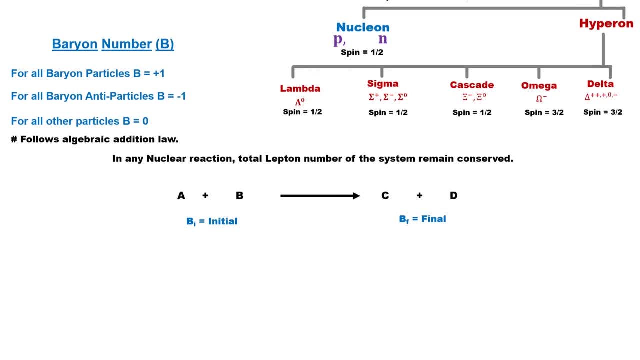 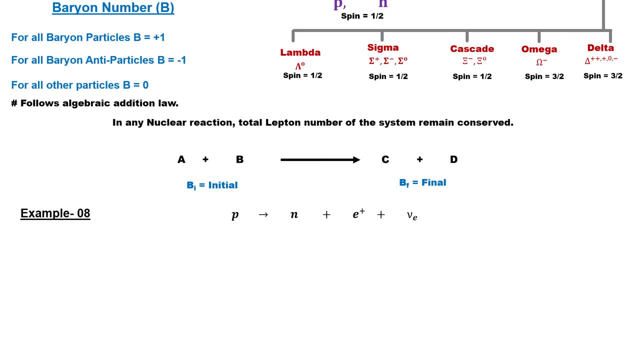 be equal to the total baryon number of the daughter particles. This is a beta plus decay, in which proton decays to neutron, positron and electron neutrino. Since proton and neutron are baryon particles, their baryon number is plus 1, while electron and electron neutrino. 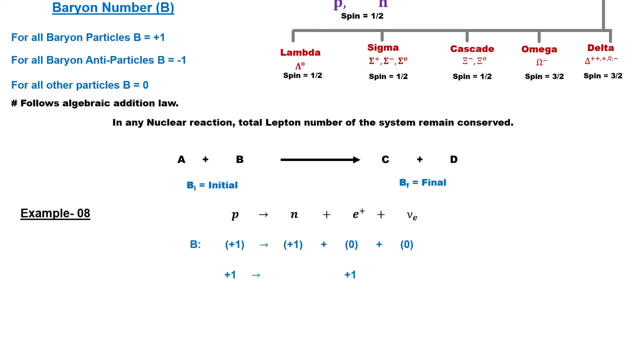 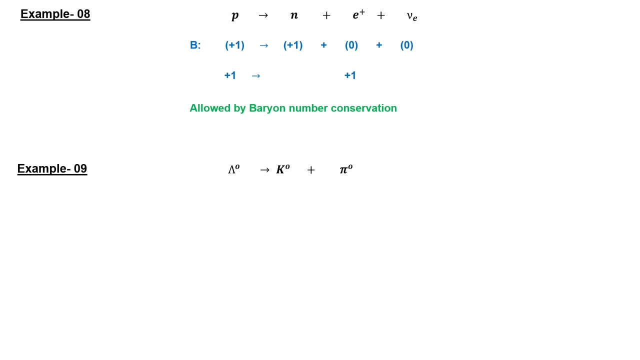 are non-baryonic particles, So their baryon number will be 0.. Since the baryon number is conserved in this reaction, this reaction is allowed according to baryon number conservation. The lambda is decaying into kion and pion. In this decay reaction, lambda is a baryon. 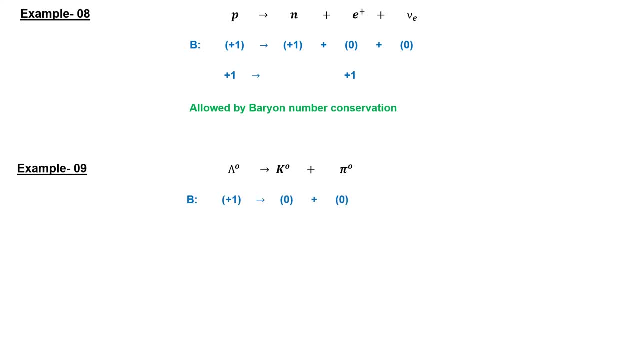 particle having baryon number plus 1, while kion and pion are non-baryonic particles having baryon number 0.. Since the baryon number is not conserved in this reaction, this decay reaction is not allowed according to baryon number conservation. 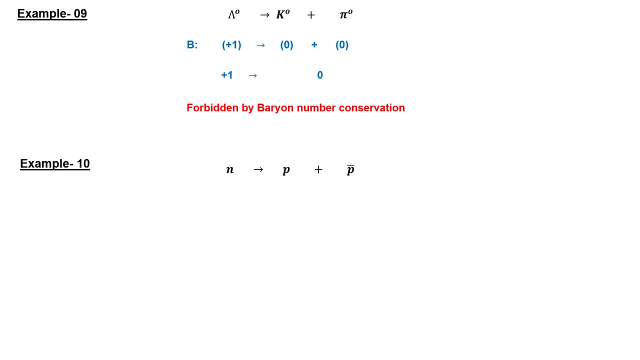 The neutron is decaying into proton and antiproton. In this decay reaction, proton and neutron are baryon particles having baryon number plus 1, while antiproton is an anti-baryon particle having baryon number minus 1.. Now, since the baryon number is not conserved in 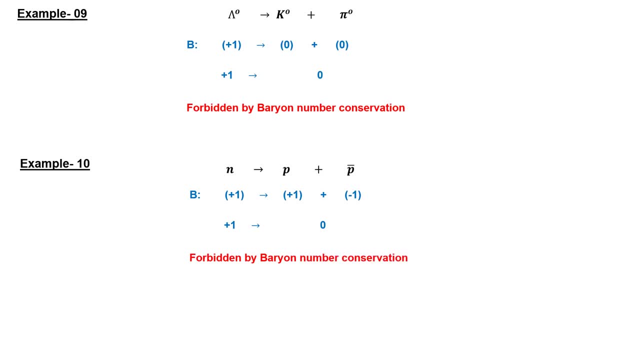 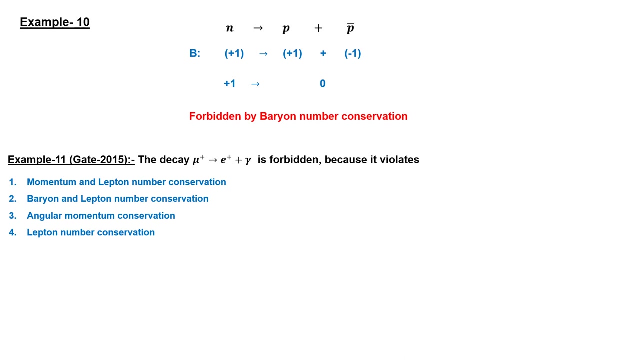 this reaction. this reaction is also not allowed according to baryon number conservation. A question was asked in GATE 2015,. this decay is forbidden because it violates. In this reaction, it has been asked that, due to violation of witch conservation law, this reaction is. 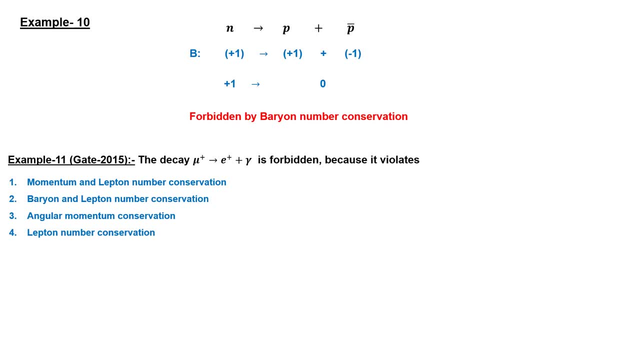 forbidden. Let us first talk about momentum conservation. As we learned in the last lecture, in any decay reaction it is necessary for linear momentum conservation that the linear momentum of parent particle should be equal to the daughter particles. Since this is a decay reaction, we can assume that the muon is decaying in rest. Therefore its linear momentum will. 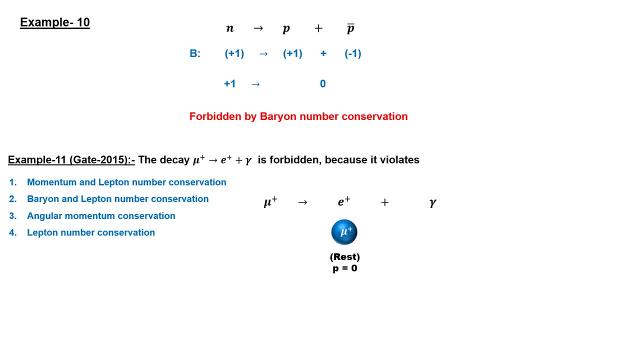 be zero After the decay. positron and photon are releasing, Since the photon cannot remain in the rest position. so to maintain momentum conservation, if we assume that the photon is released to the right side, the positron may release to the opposite left side with 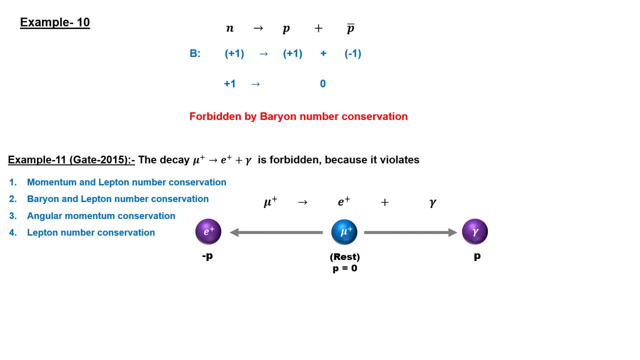 the same momentum and cancel each other's momentum, Due to which the total linear momentum of daughter particles will also be zero. Talk about angular momentum. In this question, there is no information about the orbital angular momentum of the particles, So we can assume particles in their ground state. 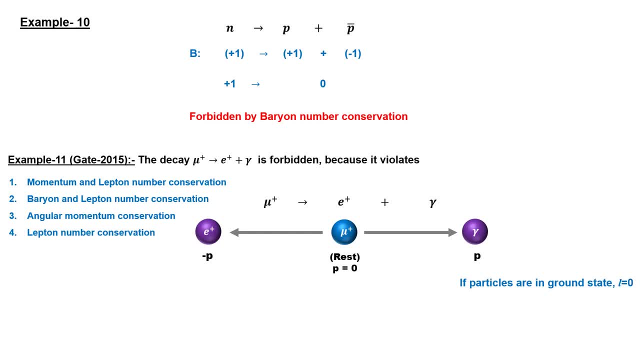 S state, having orbital angular momentum zero. That means their total angular momentum will be equal to their spin angular momentum. Both the muon and the positron are spin half fermion. while the photon is spin half fermion, Photon has spin 1.. So the vector sum of positron and photon will be 1 by 2 or 3 by. 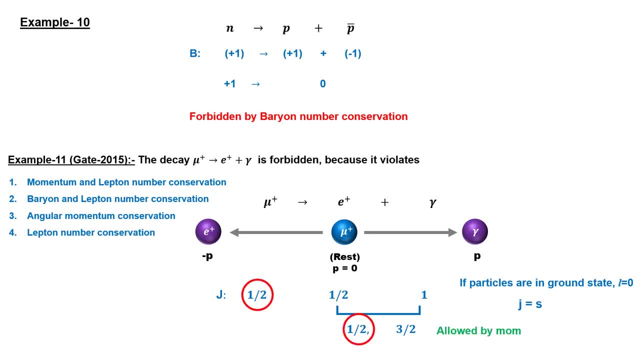 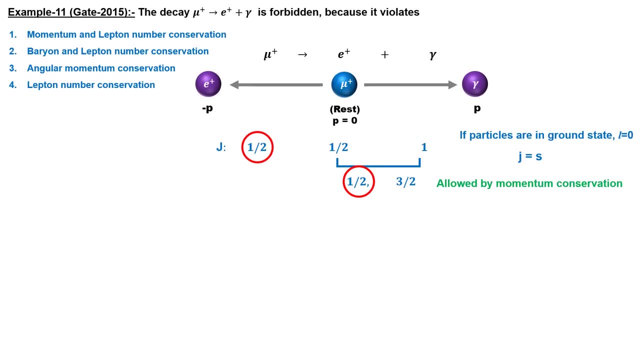 2. This matches the spin 1 by 2 of the muon. That means this reaction also conserves angular momentum conservation. Now let's verify baryon number conservation. None of three particles present in the reaction are baryon, So the baryon number is conserved. Now let's talk about lepton number, Muon and 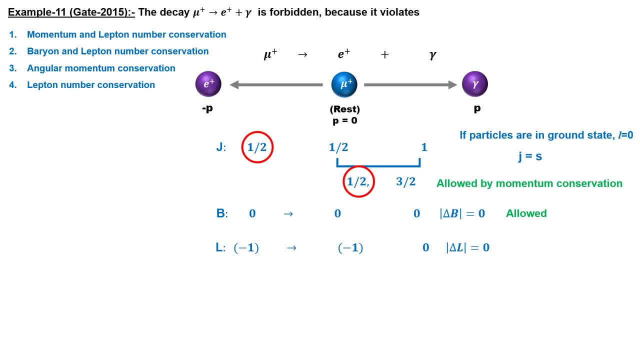 positron are both anti-lepton particles, So their lepton number will be minus one, while the Photon is a non-lepton particle, So its lepton number will be zero, Since in this reaction, total lepton number of muon is equal to the total lepton number of daughter. 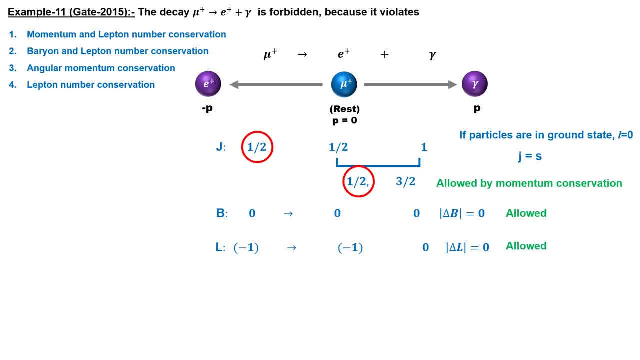 positron and photon. therefore, the total lepton number is also conserved. But as we have known, in addition to the total lepton number being conserved, the lepton number is also required to be conserved for the individual family. In this reaction, positron is present, which is a member of electron family. 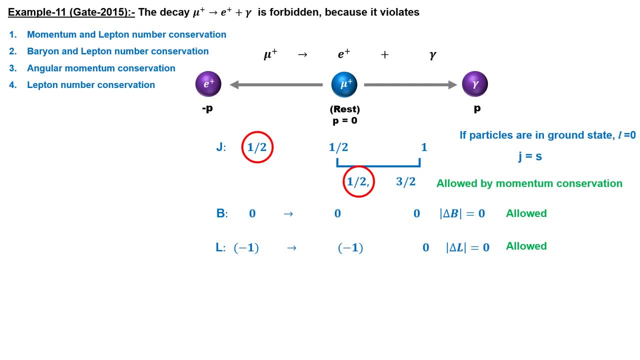 So if we verify electron number, both muon and photon are not the members of electron family, means their electron number will be zero, while positron is an antiparticle of electron family, then its electron number will be minus one. As you can see, electron number is not conserved in this reaction. 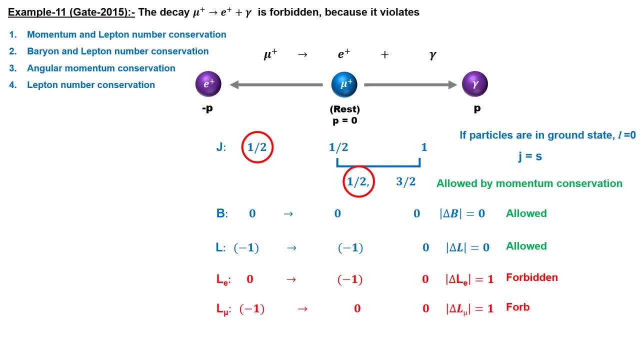 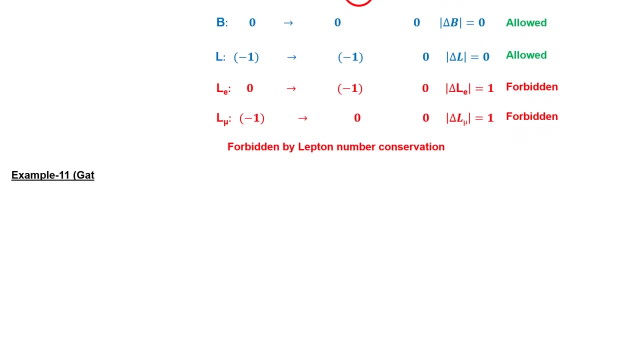 Similarly, the muon number is also being violated, Although the total lepton number is conserved in this decay reaction, but due to the violation of electron and muon number, this reaction will be forbidden according to lepton number conservation. A question was asked in GATE 2019, consider baryon number and lepton number conservation. 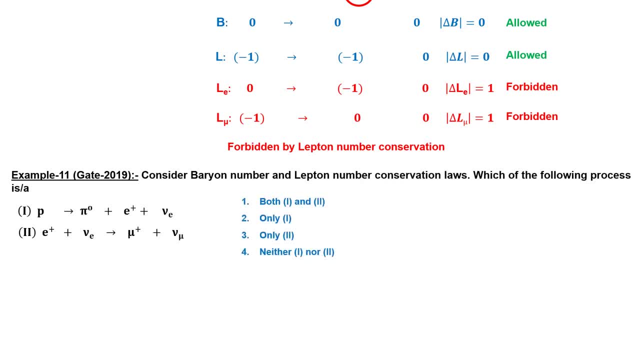 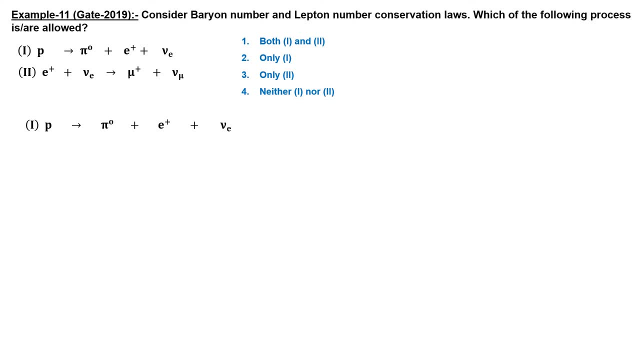 laws. Which of the following processes are allowed? First, let's verify the lepton number. Both proton and pion are non-leptonic particles, so their lepton number will be zero, while positron is anti-lepton, its lepton number is minus one. 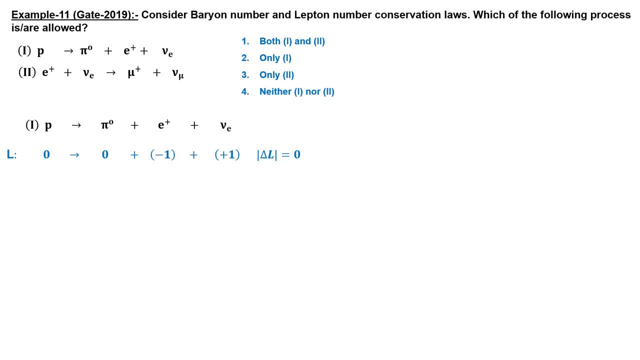 And electron neutrino is a lepton particle, its lepton number will be plus one. As we can see, the total lepton number is conserved in this reaction. But this is not enough. we need to verify the lepton number for individual family, as 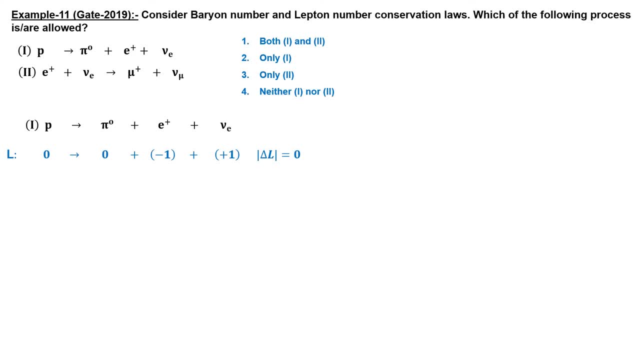 well, In this reaction Only members of electron family are participating, so we need to verify the electron number. The electron number for proton and pion will be zero, while positron's electron number is minus one and neutrino's electron number is plus one. 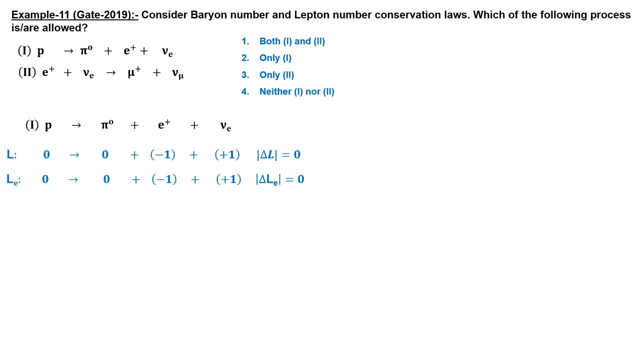 Since electron number is also conserved in this reaction, that means this reaction is allowed according to lepton number conservation, Talking about the baryon number. in this reaction, the proton is the only baryon particle having baryon number plus one, while for the rest of the particles baryon number will be zero. 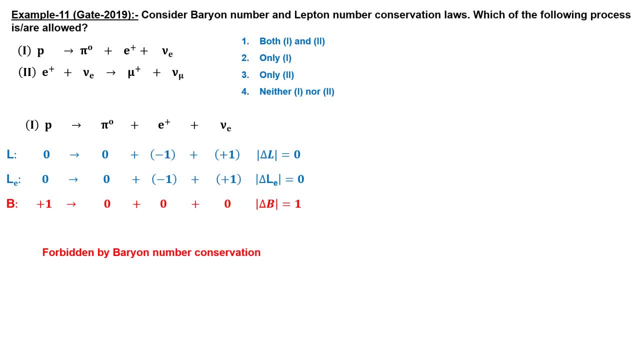 As you can see, baryon number is not conserved in this reaction. Now let us verify both these conservation laws for the second reaction. In this reaction all particles are lepton. Positron and muon plus are anti-lepton, so their lepton number is minus one, while both 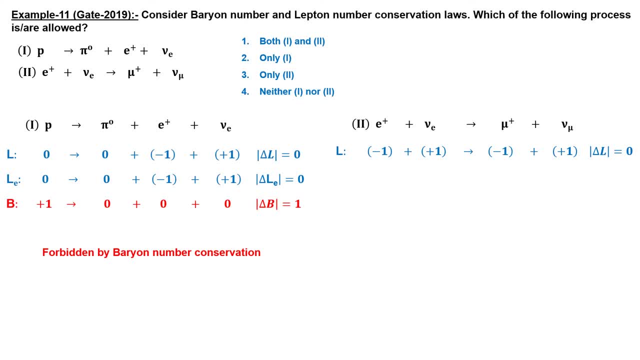 neutrinos are lepton particles. their lepton number will be plus one. Therefore, In this reaction, the total lepton number is conserved. Talking about electron number, positron and electron neutrino are the only members of the electron family. 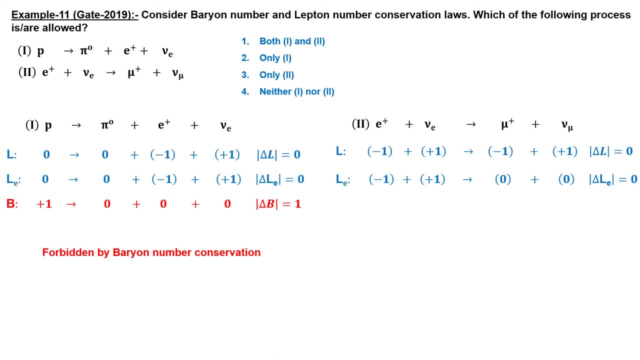 Therefore, in this reaction, the electron number is also being conserved. Similarly, muon and muon neutrino are the members of the muon family, having muon number plus one, Since the total lepton number is conserved in this reaction as well as the lepton number.